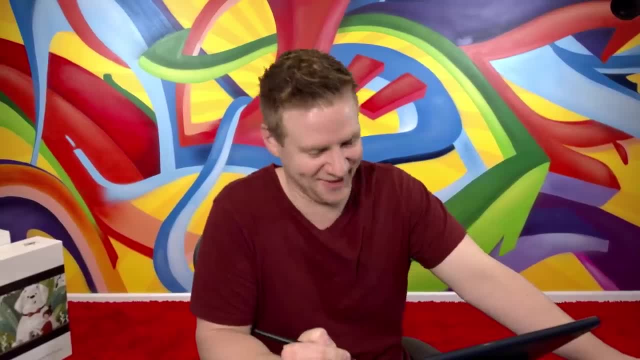 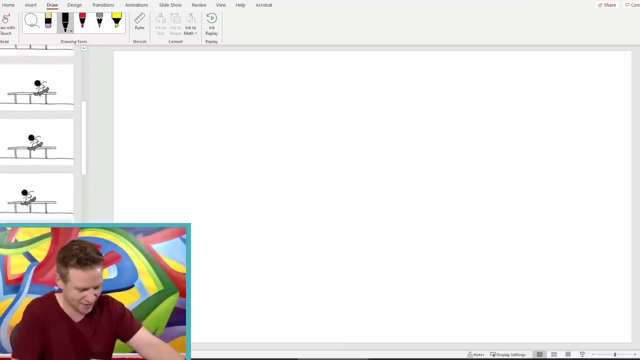 again Go back here. It's a very tedious process. Copy Paste Next frame: Select Grab Move Place. Select. Copy Paste Next frame. Go back. Select Move Resize Place- Select. Copy Paste Next. 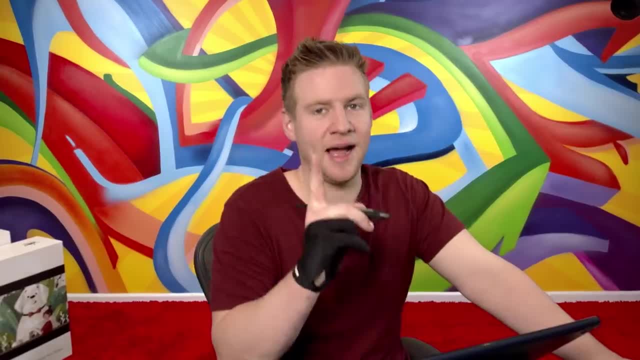 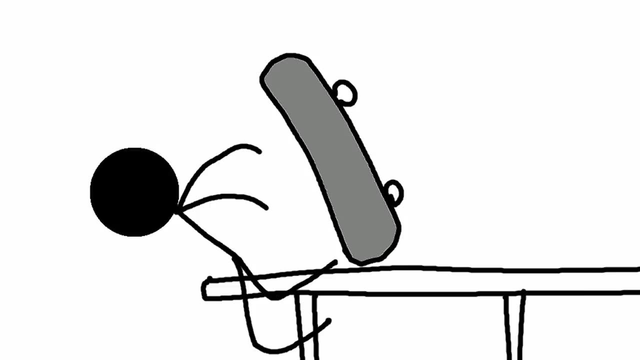 frame: Select Move, Resize Place, Select Copy, Paste. Next frame: Undo and select Delete. So I'm going to animate. He slipped and the skateboard's flipping up this way: Boom, Select Copy. Boom, That's some good motion Skateboard's flying off here. Select Copy Paste. 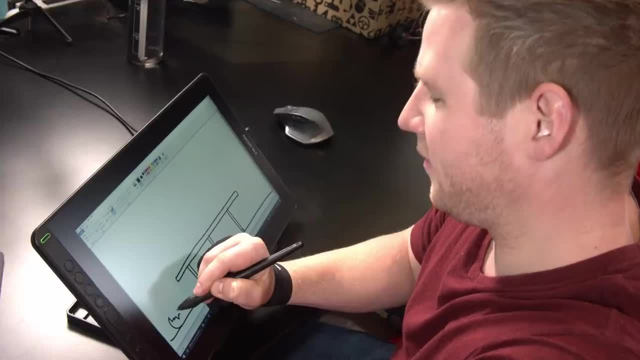 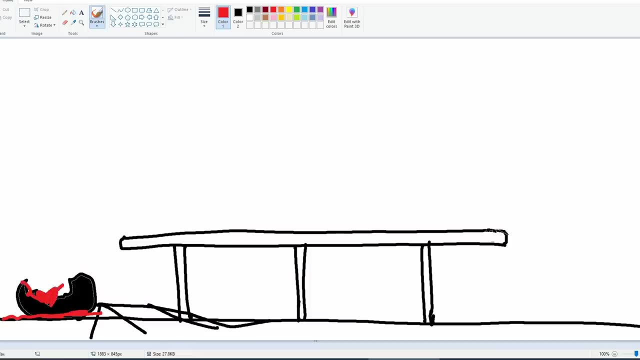 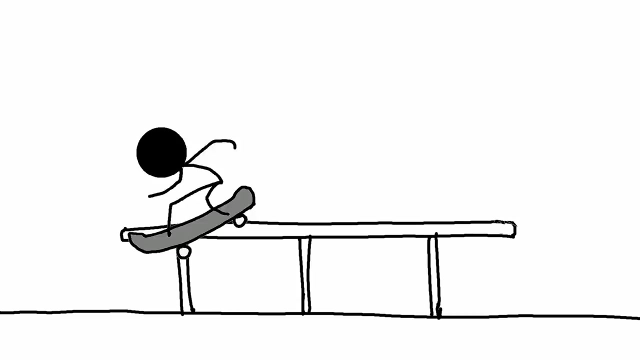 Next frame: Little motion lines there Fly off screen And the final beautiful frame We've got the stick figure's head cracked open. Just a real old mess of blood and gore. and grab some pink. There's some guts out here. This was my childhood. I mean, that's pretty good, but it's manually I. 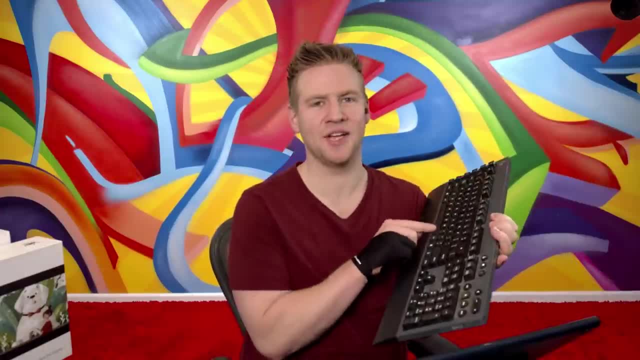 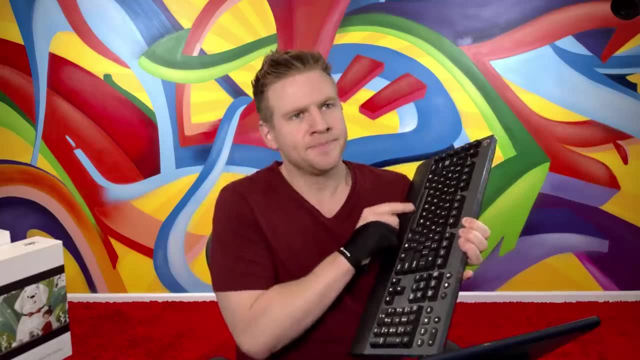 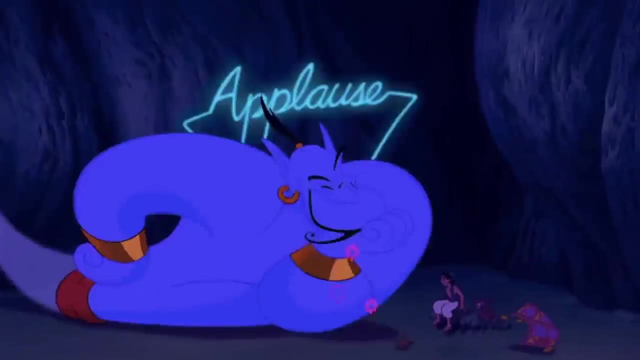 mean we don't want to do that. That's not an animation. I mean, if every time you watched Aladdin you had to, You probably wouldn't watch many animations. So let's figure out how to automate this, And I know. 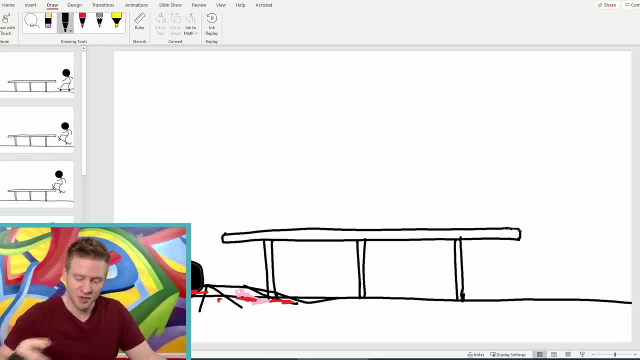 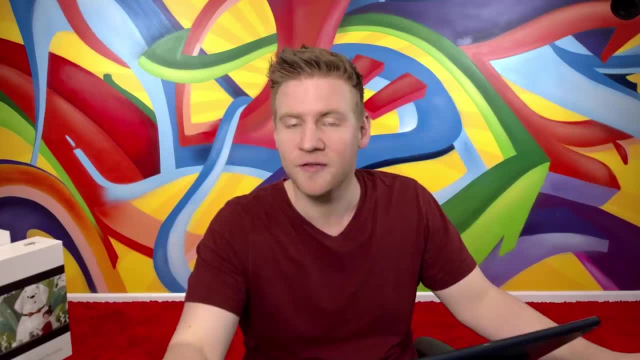 I figured out this in the past. In fact, just for context, I didn't just do this, This was the style of my first ever animations. But once I'd figured this out, I went crazy And I full on animated like a hundreds of frames Mortal Kombat. I didn't just do this, I did this. I did this, I did this. 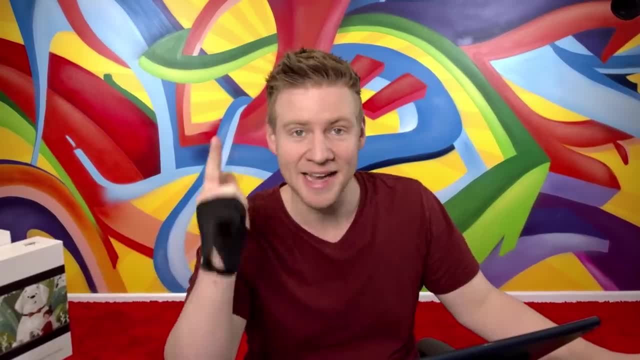 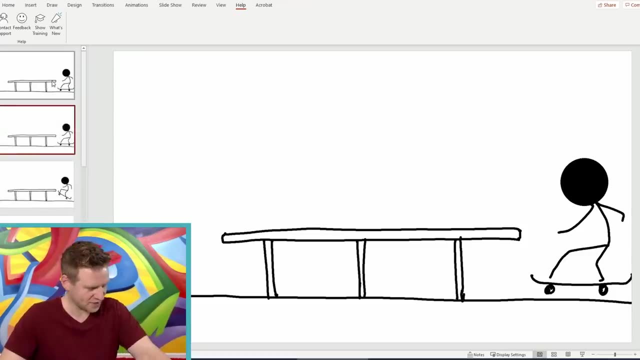 I figured out how to add music, I figured out how to add sound effects, And I'm going to do that again today. But let's start off by figuring out how to get it to play itself. I mean, here's a thought. Let me duplicate the first slide. Can I crop There? we go Paste Send to the back. Look. 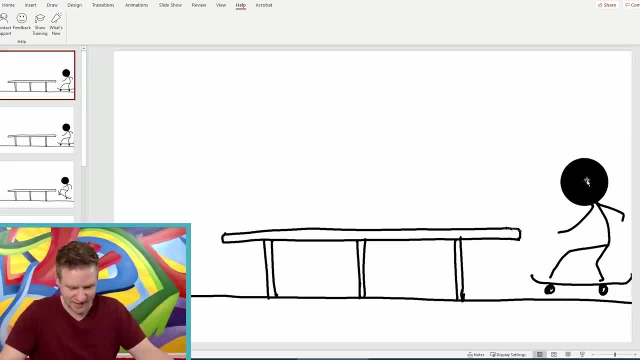 at that. I've got two separate things in the exact same position, except this time animations. He's going to come in from the right. Hey, All right, What's next? I want to auto frame thing. Advanced slides automatically is an option. 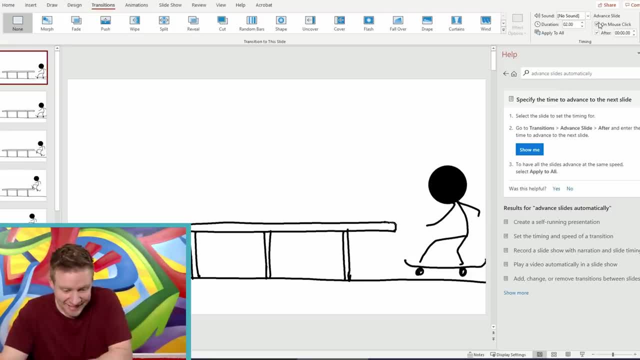 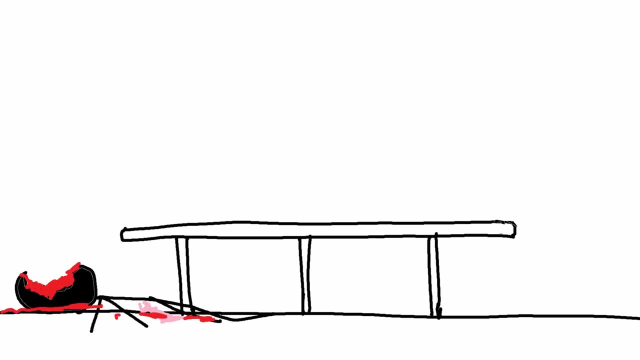 On mouse click After. There it is. That's what That's it. That's it. Ooh You ready. It worked perfectly. This is so much better than I expected. Oh my God, I could do so much with this And I'm. 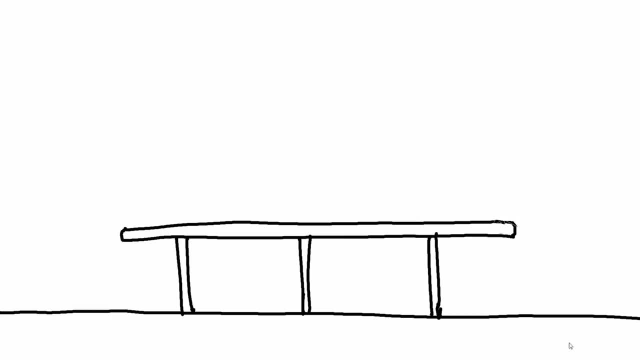 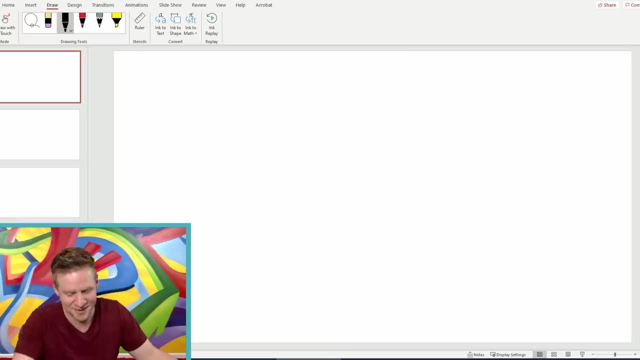 going to. They come with sound effects. Push, sound, What's that sound like? It's all right actually. Then on this frame, let's play one of these. Here we go. You ready, I am mind blown. You can actually animate in PowerPoint. I can make cool stuff in this, And so can you with a. 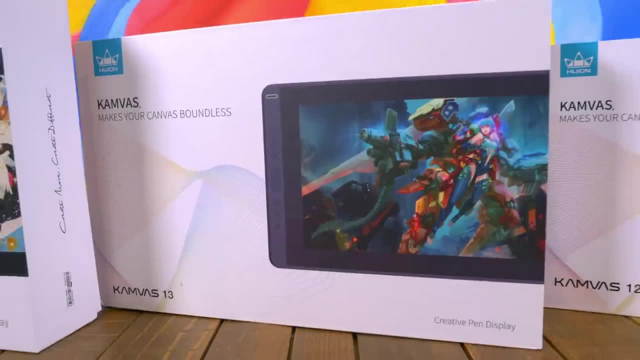 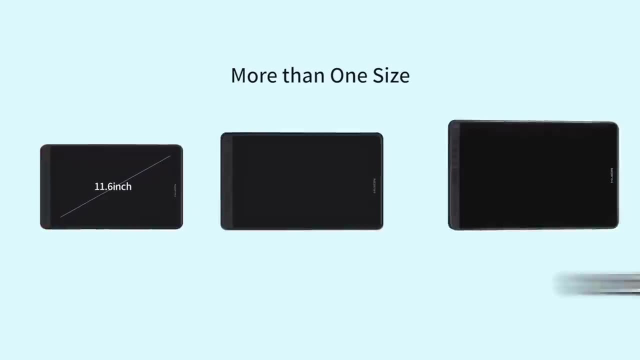 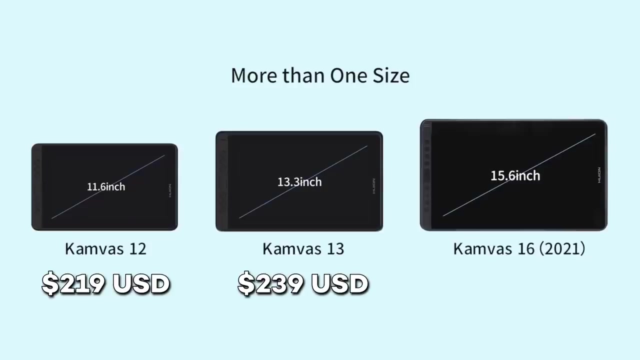 brand new lineup of Huey on canvas tablets to pick from. The canvas 12,, 13, and 16 tablets are the most affordable pen display tablets you can get. The canvas 12 has an 11.6 inch screen for only $219.. The canvas 13, 13.3 inches for only $239.. The canvas 16- 2021 edition has 15.6 inches of screen. 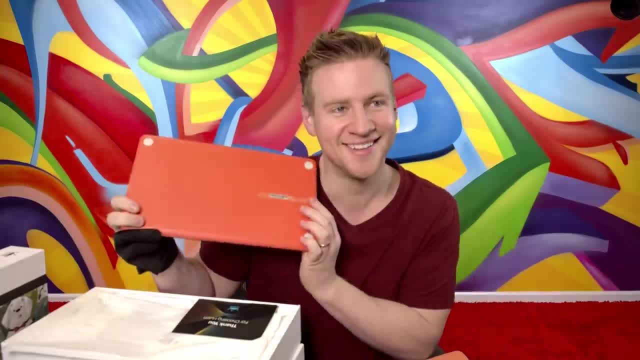 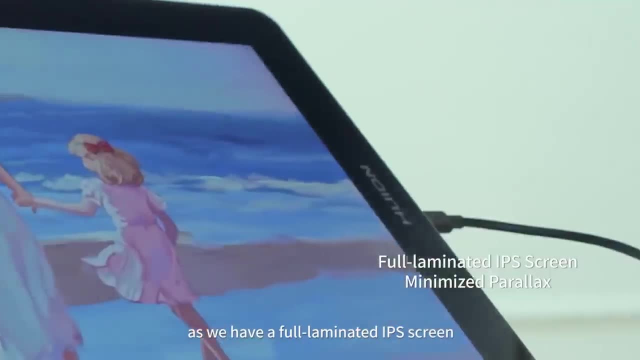 for only $399.. And oh, by the way, it comes in different colors. It comes in different colors. You need to be able to express yourself, baby. 120% sRGB, 92% Adobe RGB, 88% NTSC color gamut, The. 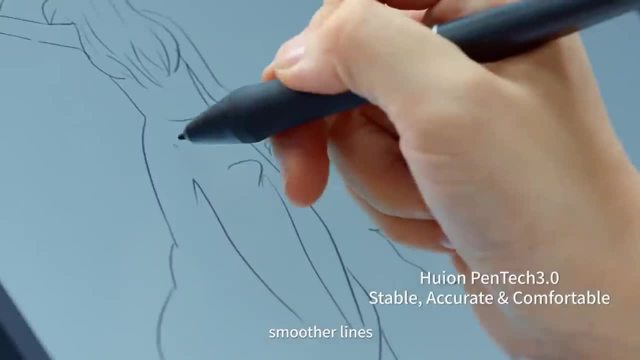 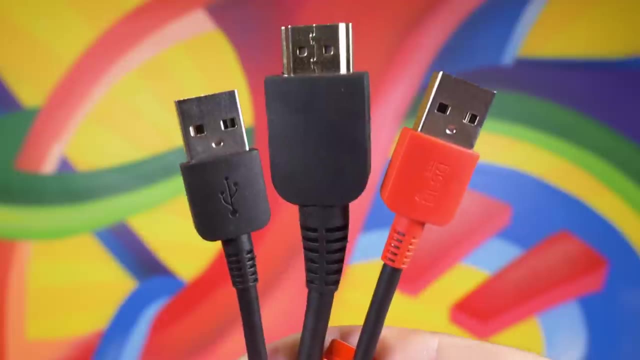 Pentek 3 stylus has 8,192 levels of pressure sensitivity. They all have tilt support and full HD screen resolutions. They all have customizable keys and loads of customization settings. They come with a three-in-one cable, so you don't have any clutter And they all plug. 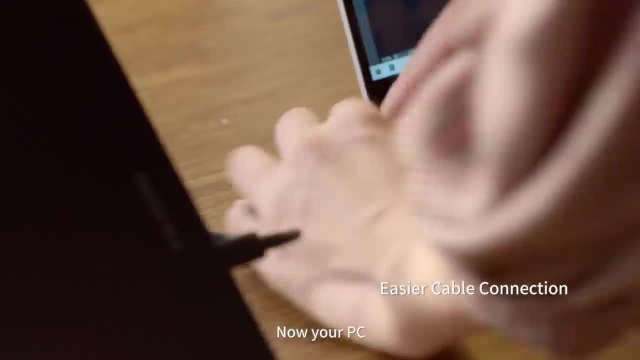 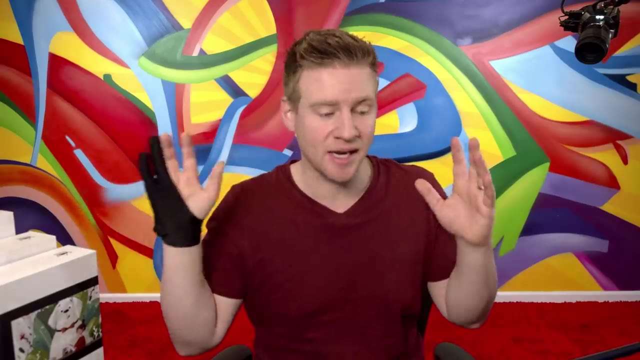 in with USB-C, either into your Mac or PC or into your Android device. Many laptops can power the tablet directly with a single USB-C. You can power the tablet directly with a single USB-C. You can power the tablet directly with a single USB-C cable, which makes these tablets incredibly. 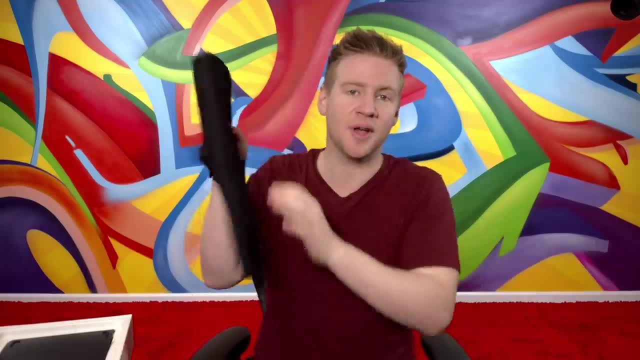 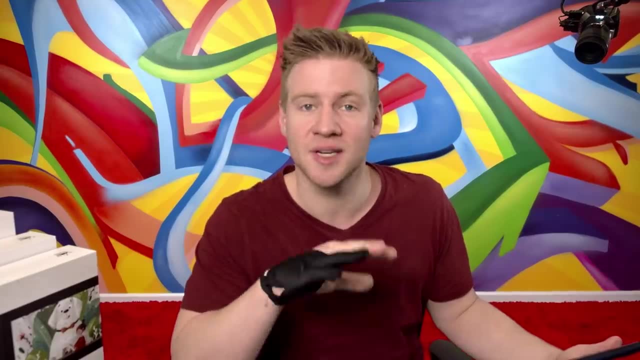 portable. Fit it right in the back with the satchel that you take with you on the go, or fit your professional, very, very portable tablet in your backpack and take it wherever you want. The links are all in the description, as well as all the details. Go check them out for yourself And we're 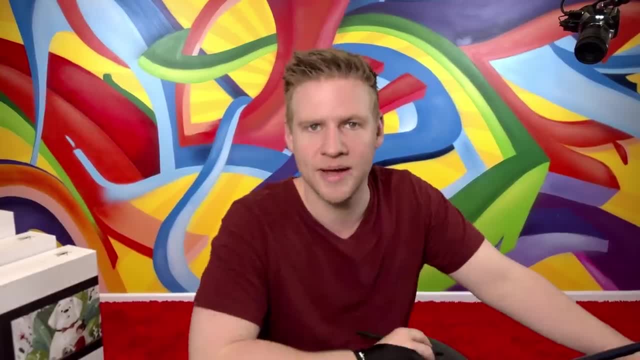 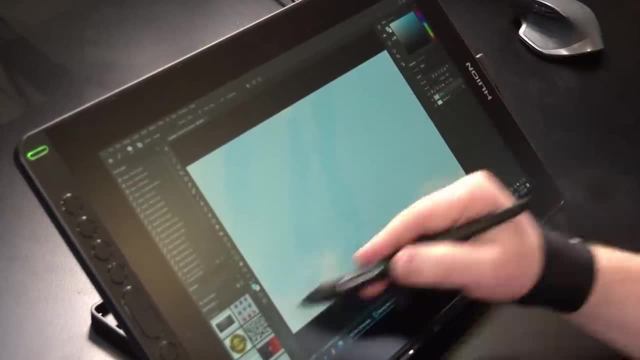 going to put some of that pressure sensitivity to the test and we're going to make a Mortal Kombat fight. We're opening Photoshop, not paint. We're taking things to the next level. I'm going to recreate to the best of my ability the Mortal Kombat style stick figure animation to the death. 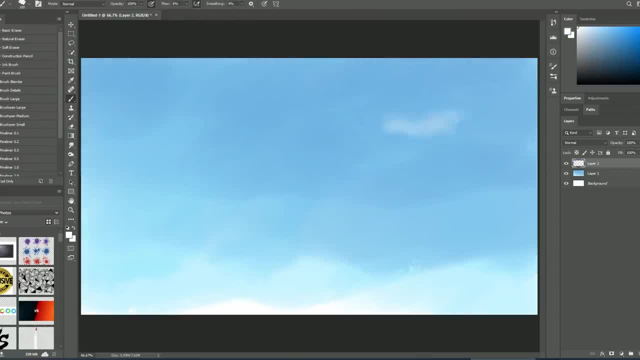 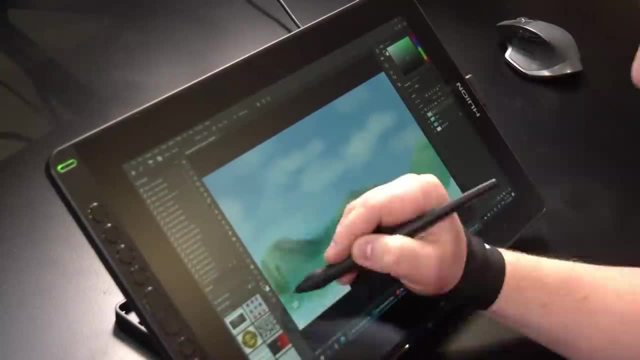 that I made when I was 12.. I remember the background I did was basically just like a grass, like ground point. I'm going to take that a few levels beyond. Let's add some distance, some mountains. Last but not least, we have our 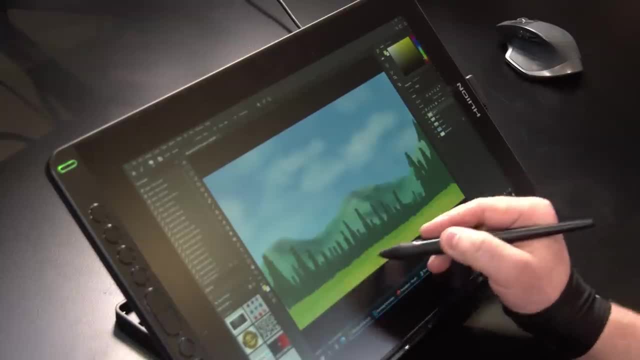 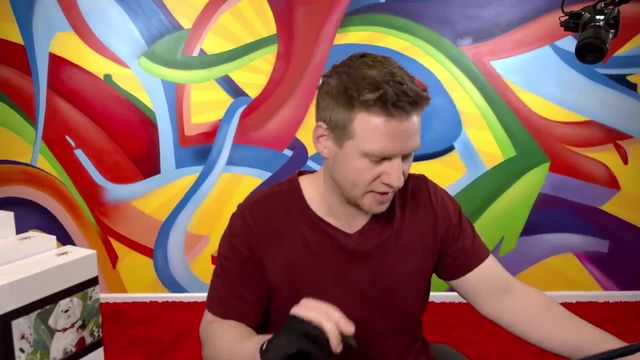 ground a little bit of texture on the edge. It looks a little bit grassy. It's nice. It's a beautiful, sunny summer day. What could our characters possibly want to do more in this beautiful environment than fight to the death? Bring our background in here. All I need to do. 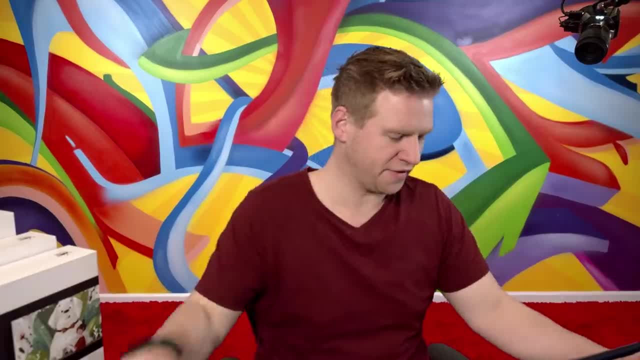 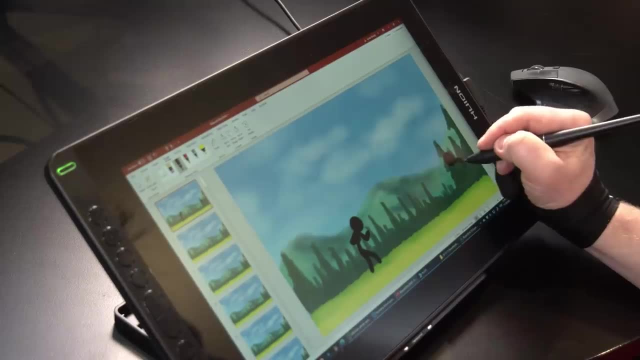 is copy and paste. Let's start off with a hundred frames. Let's draw our first head, something fairly symmetrical On the left. here. he's ready to fight, He's standing there and this guy, he's going to be running in, He's going to charge him, I mean. 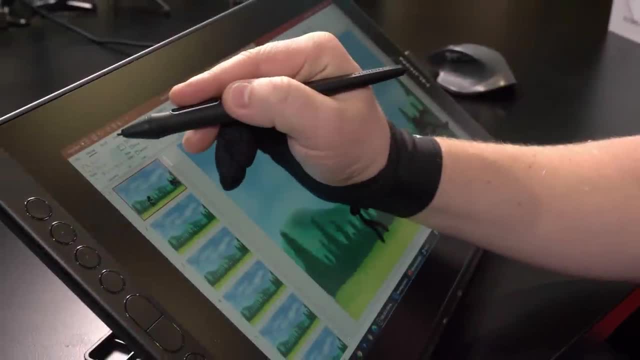 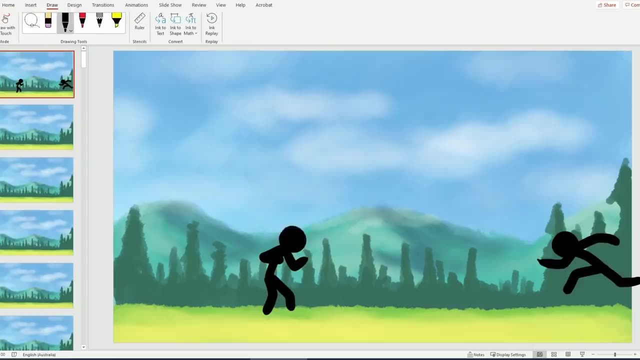 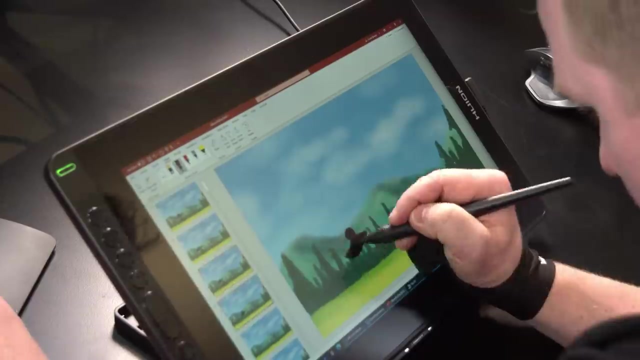 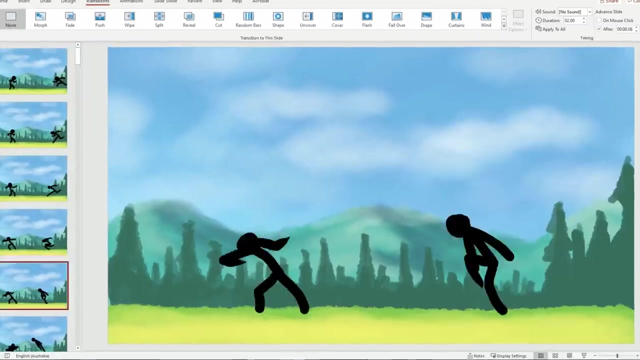 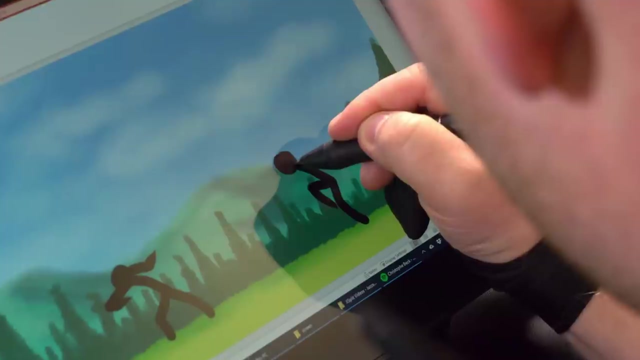 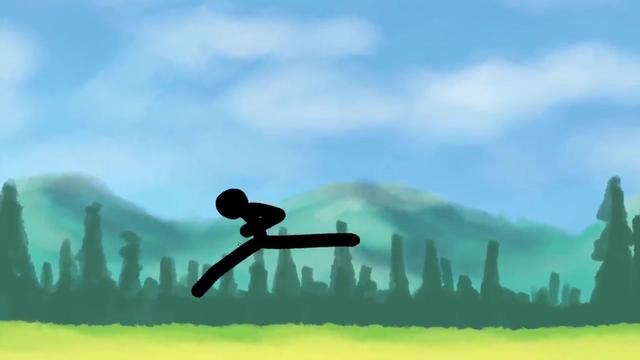 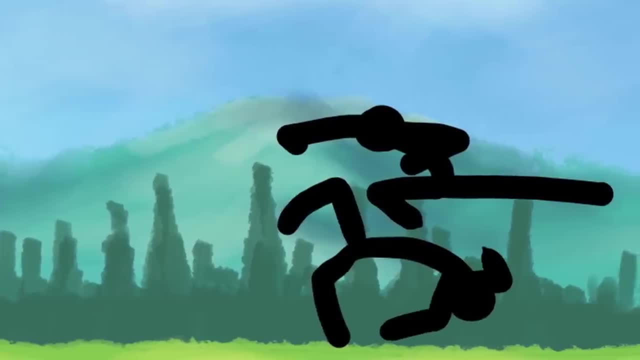 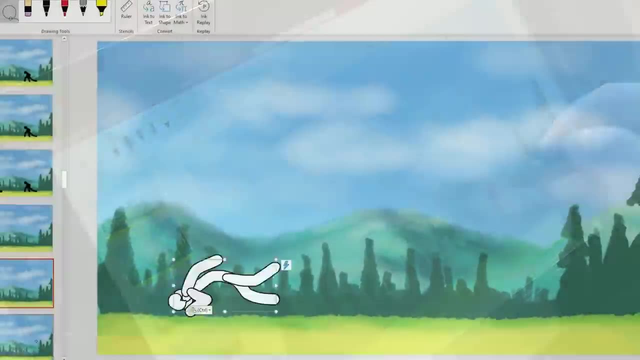 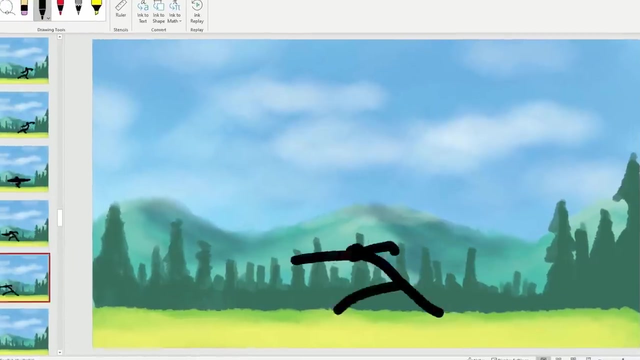 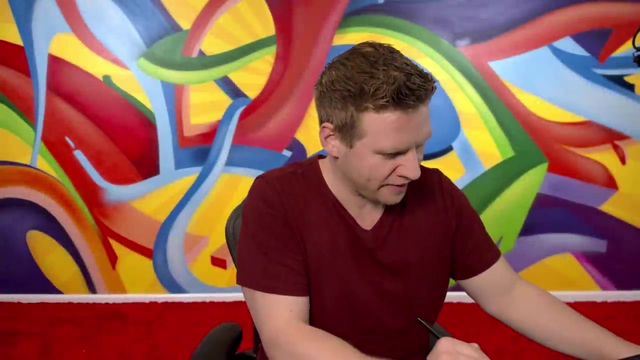 I guess I'm I get to last. get it done, never going back. We don't never going back. get it down, never going back. No, Get into town Going All right now I think I have an animation. 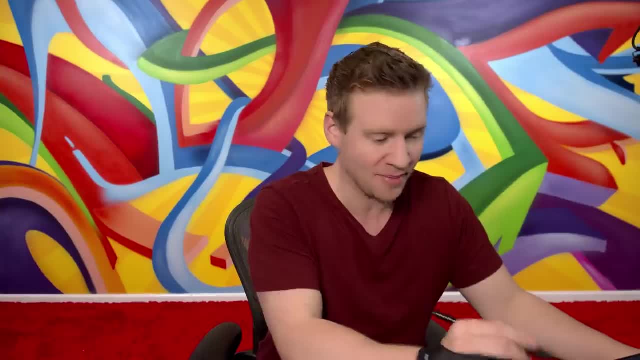 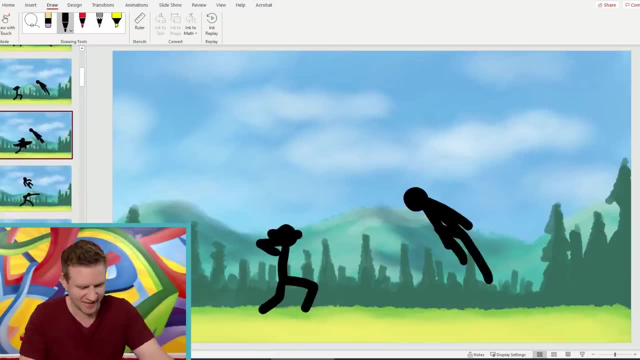 It spans 87 frames and it should loop. Now I'm not gonna play it yet. I need to add some finishing touches, starting off with blood, And actually there's not a lot of impact. they actually sort of dodge each other a lot. 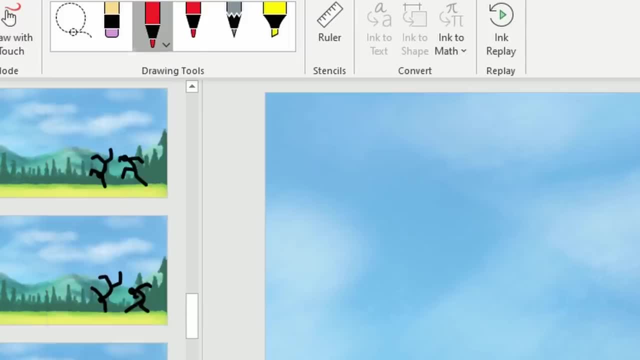 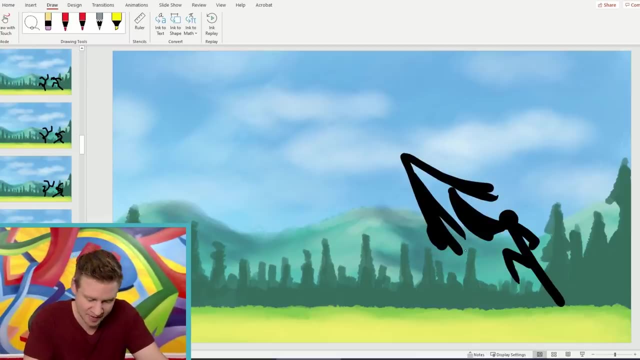 Here's one here. there you go, okay. so let's add some blood red, let's bring our thickness down. We have an impact splat here and then the next few frames. The trick with blood is you want the start frame to be where the blobs sort of go out. 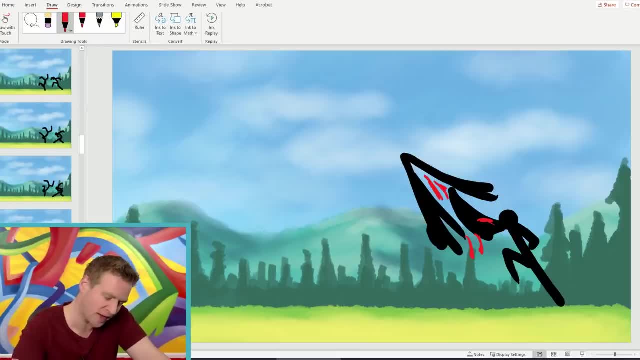 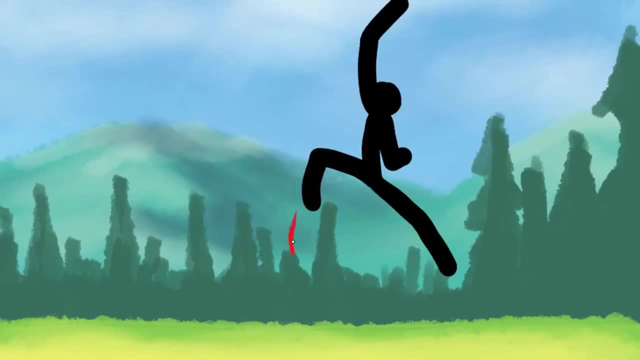 from. The temptation is to sort of go along with it, but you sort of have to do both. They have the impact splat, which has to happen where the impact was, and then there's sort of like a trail, And the trick is that you just pick one dot and you just trail it through until it's completed. 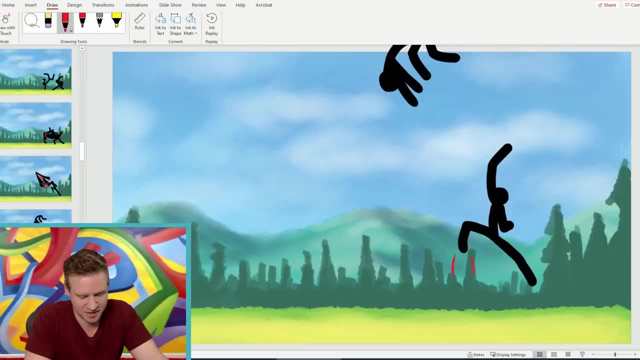 And that way you just sort of go back, pick the next bit. there's my next bit: just continue the trail Back. continue the trail, And that's how you get a really dynamic splat. There's different kinds of blood. 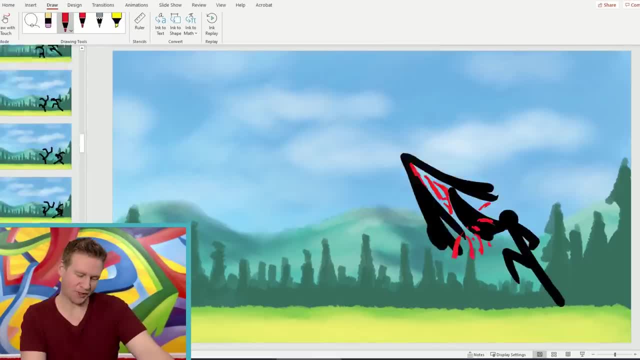 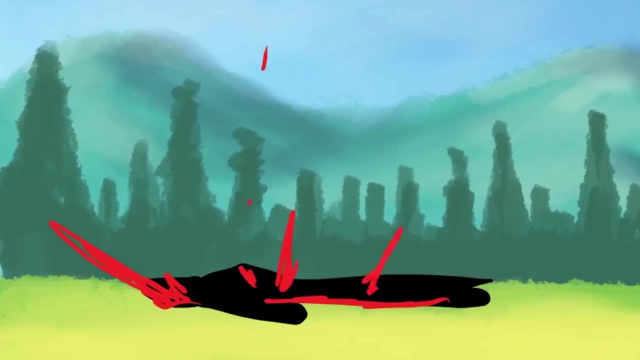 We've got the, we've got the splat that we did, and then this one's a bit of a mist. Look at that, There we go. That's good, That was good blood. Your point of impact always has to be nice and nice and aggressive. 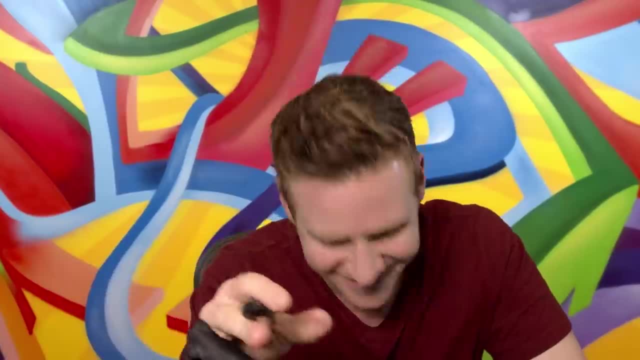 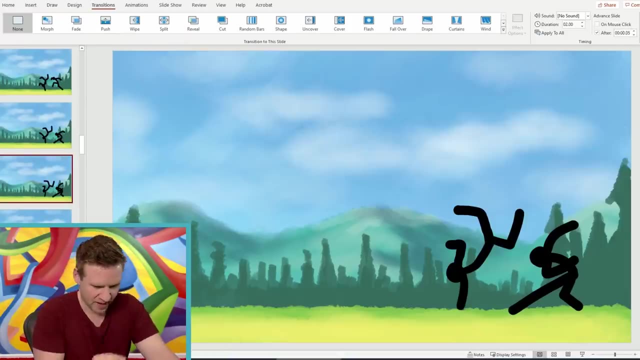 Would you guys be interested in a how to animate blood video? We're going to want to add frame timing. I want some frames to hold a little longer. Let's go 0.5.. I think for the impact there that should have a little extra. 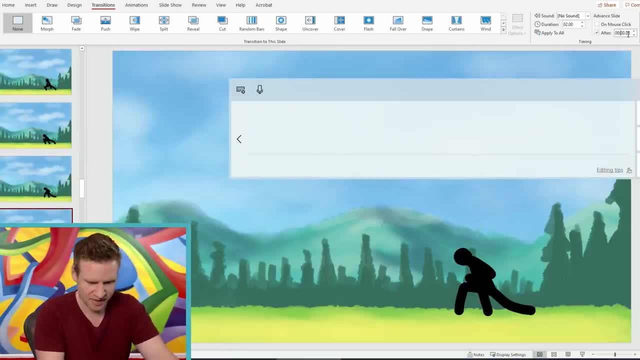 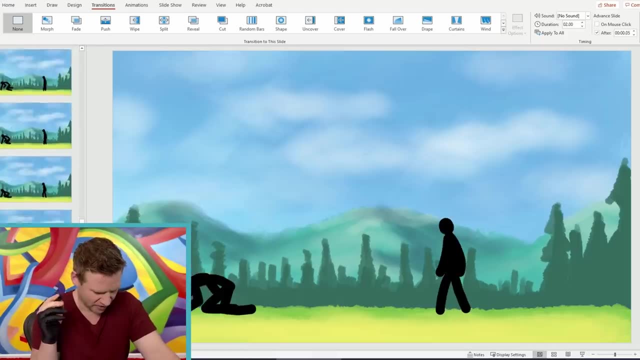 That should have a little extra love too. He should probably just be there chilling for a little bit, So let's give him, give him- two seconds standing still there before the dude falls Boom, And then they're both in a resting position here. 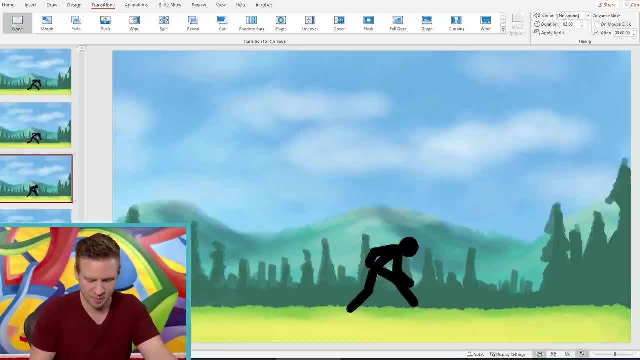 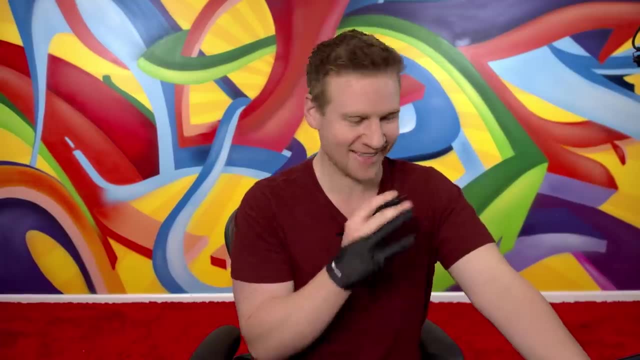 Give that three seconds, All right. I think I've got my frame holds. Let's play and just see how the timing is. There's the loop. The pauses are a little awkward, That's okay. That's actually really good, All right. 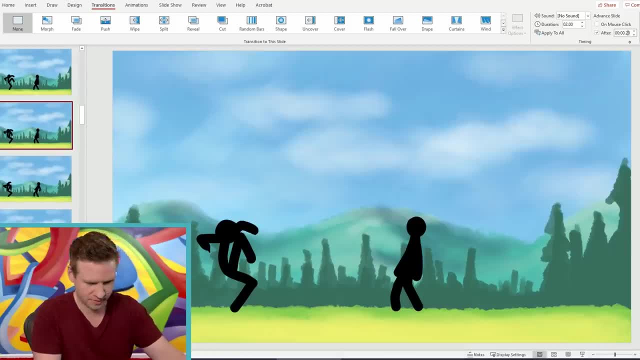 Little adjustment And then we're pretty much there. Then we just got to add sound effects. Let's go 0.2.. That's actually good. That's actually really good. All right, Sound effects time. Oh my God, Sound effects. 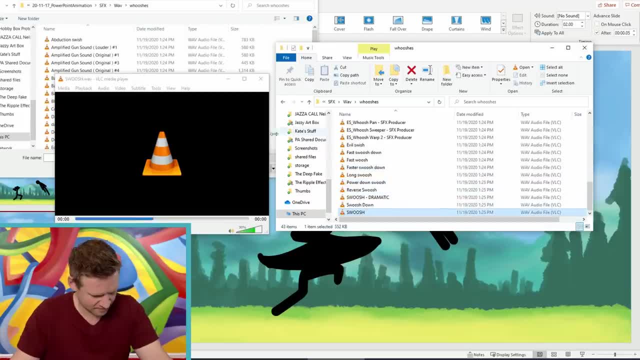 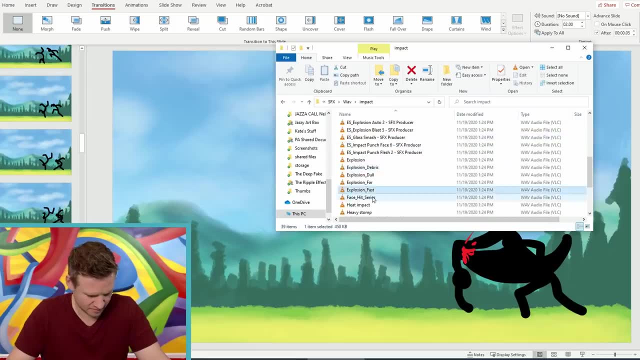 What are our whooshes like? There you go, There's a good one, Boom Down, All right. There you go. That's pretty good for there. Here's our impact. We need something chunky here. What's voice? 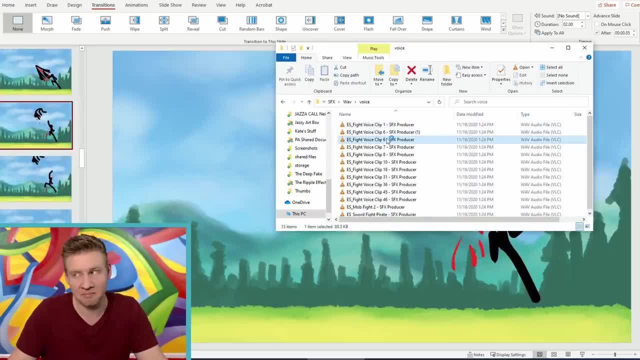 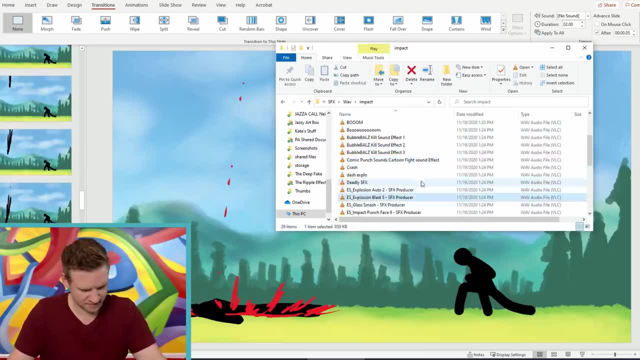 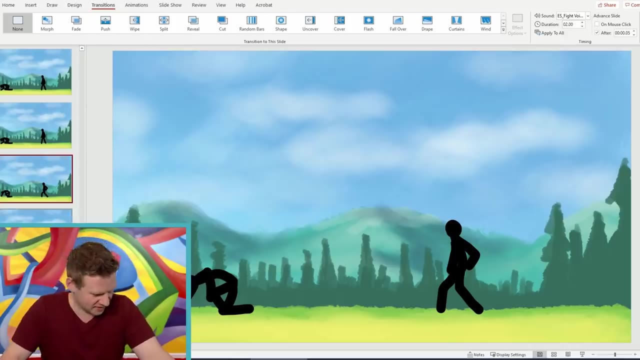 Yeah, All right, We need some. we need a good impact for this. bit Feels pretty right, That's good. We need a little bit of a wind up, That's good. We need another shock voice, That's good. 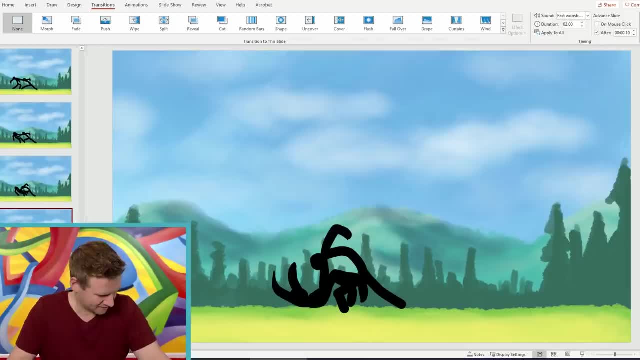 Big throw whoosh. All right, I think I have sound effects in place. I have no idea if this is going to work or what the timing is going to be like, but we're going to experience it together for the first time. Oh my God. 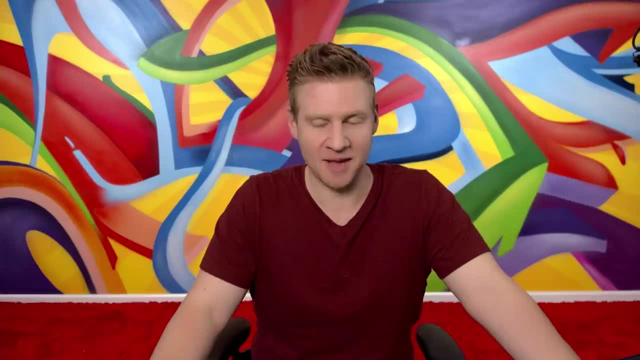 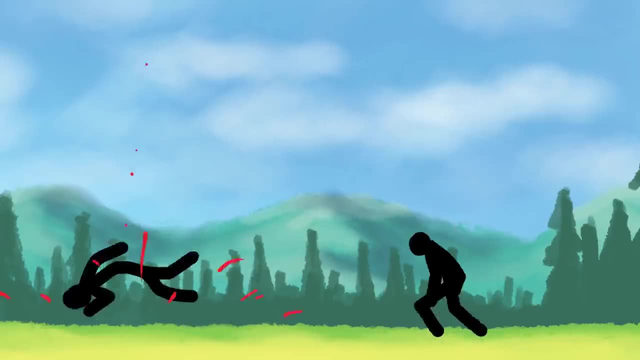 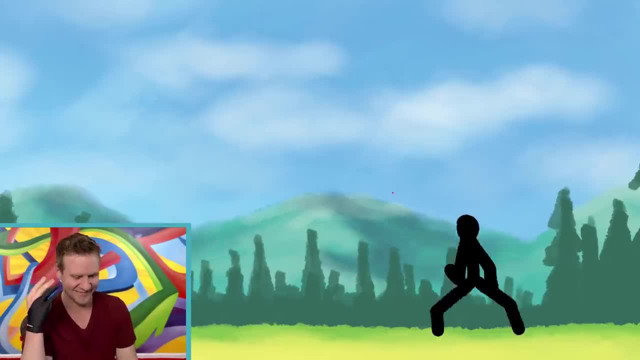 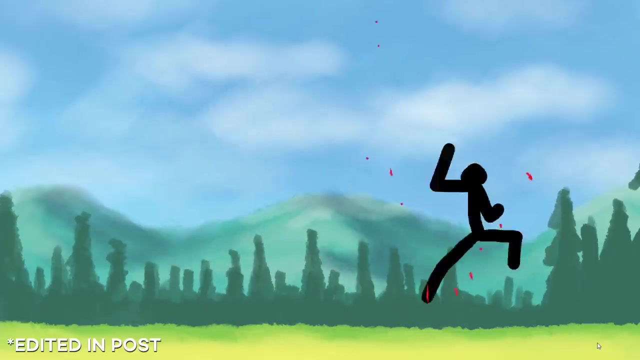 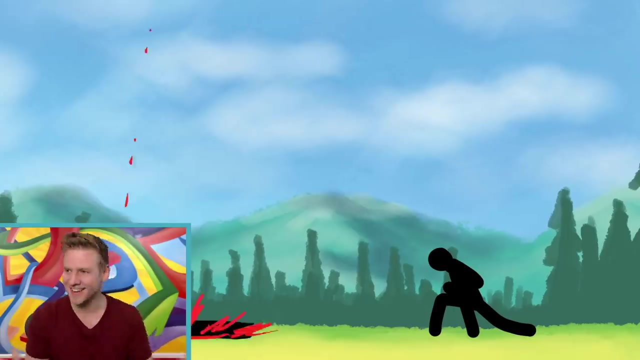